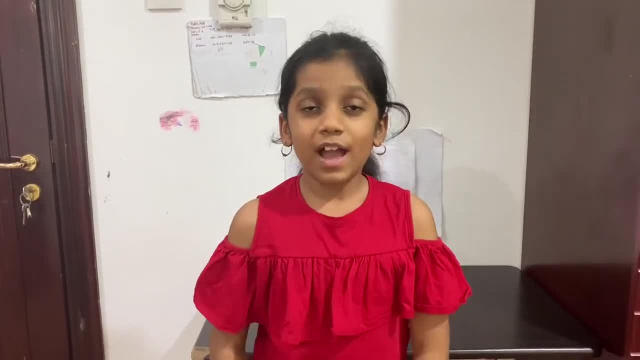 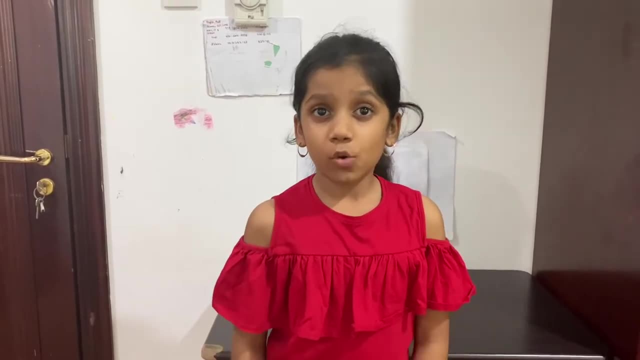 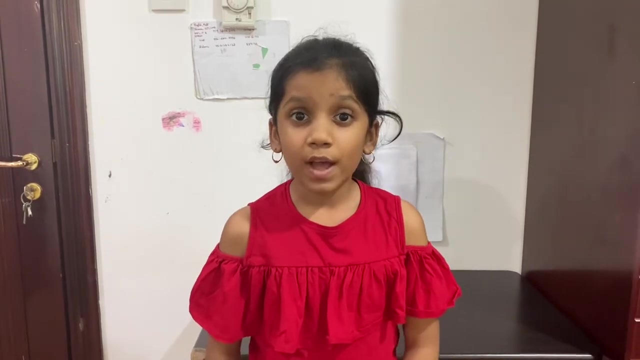 Hello everyone. I am Madiha from grade 4F and today I am presenting sustainable transportation. Cities around the world are growing rapidly. More than 70 percent of world population are living in cities. Do you know? 75 percent of global energy consumption occurs in cities. and 85 percent of gas emission causes global warming from our cities. Most of the developments in cities are not sustainable and showing no mercy on planet resources. Then how can we avoid air pollution? with sustainable transportation. Sustainable transportation means that the transportation that is green and has low impact on environment. 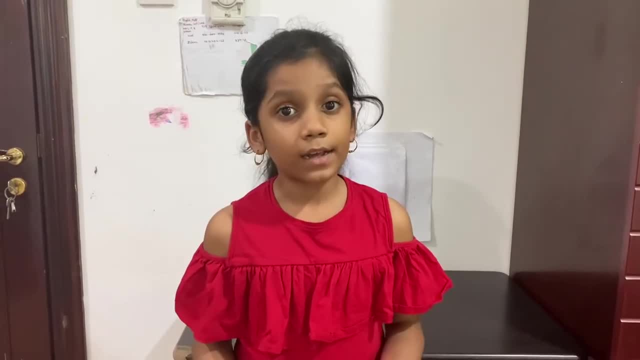 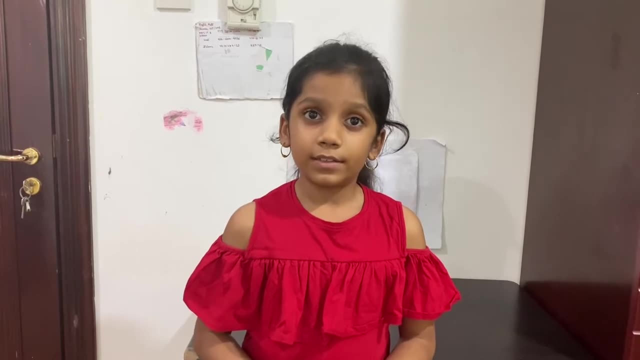 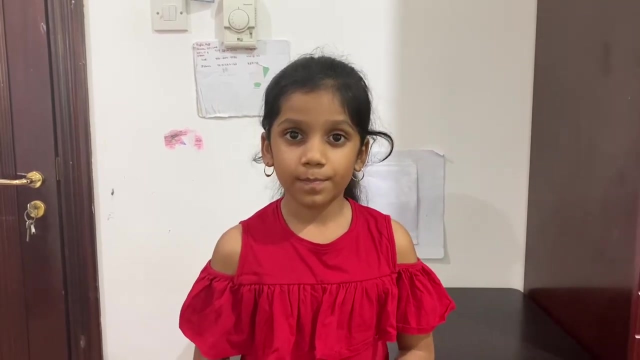 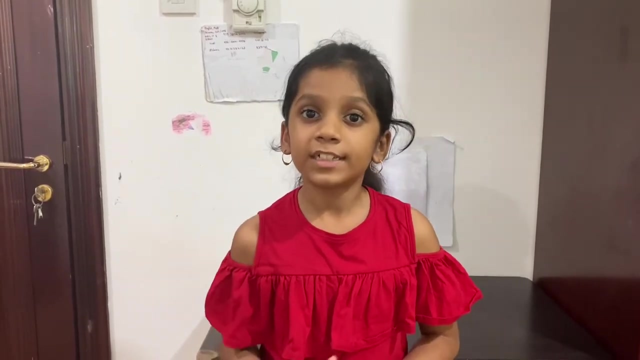 Some examples are walking, cycling, public transport, car pulling, car sharing, electric, bike and hybrid vehicles. Then how can we promote sustainable transportation? Plan the cities in such a way that to live a healthy and happy life is found within a 20-minute public transport, and also making public transport cost effective. 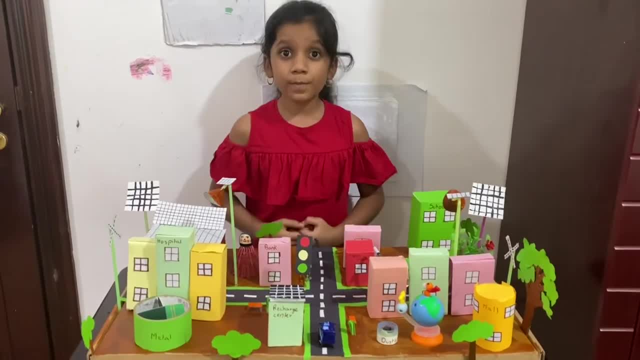 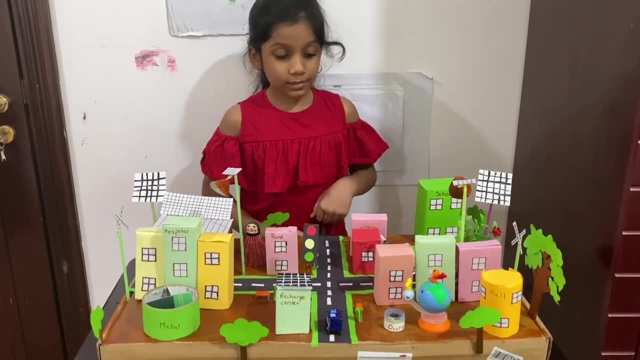 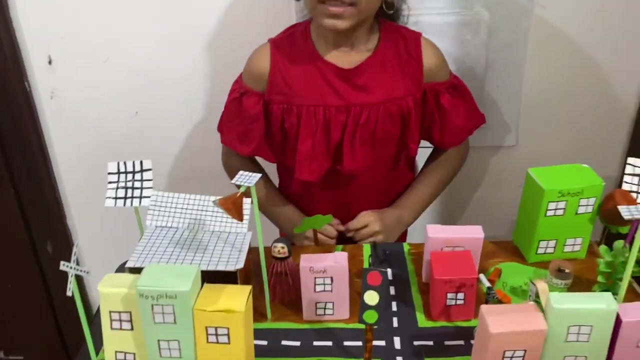 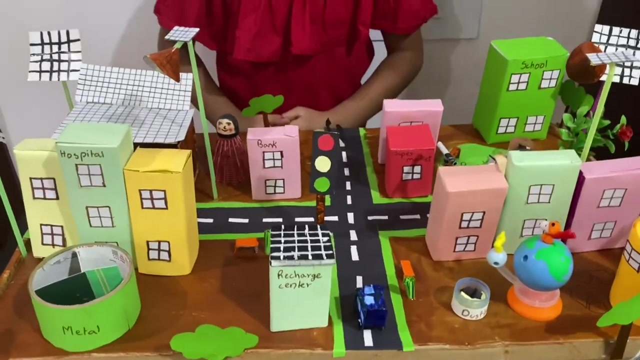 The first example is my smart sitting model. I used cardboard medicine boxes, glue gun and straw to make this. There is a supermarket, bank, school, mall and a hospital. There is also a recharge center that recharges the electric cars and there is a solar panel on top of it. These are solar panels and windmills. 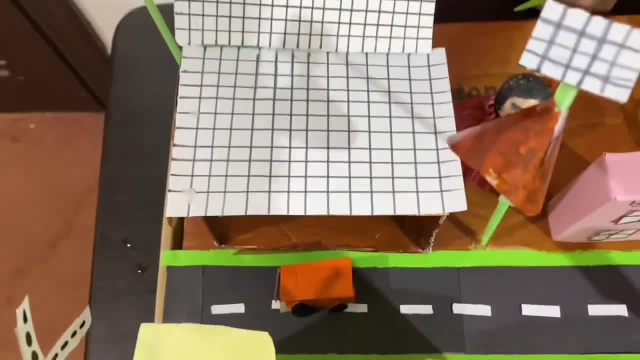 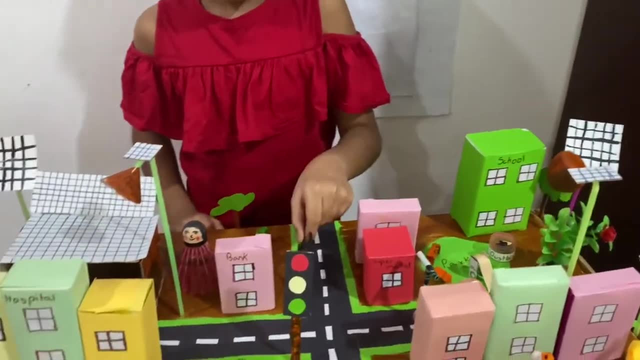 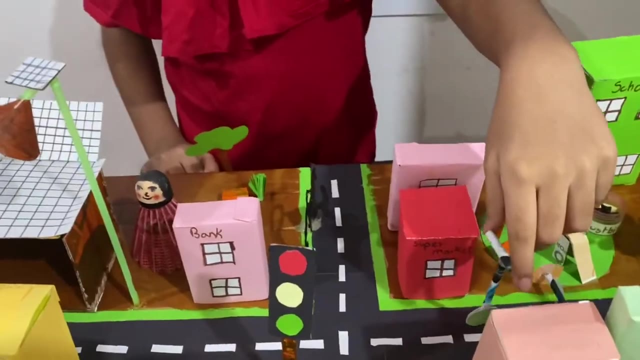 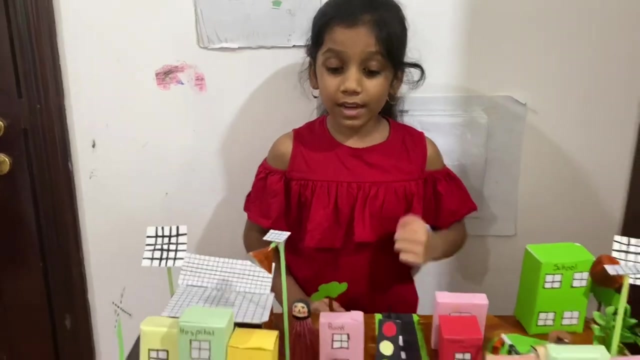 This is a bus stop. there is also solar panels on top of it and the street lights are also having solar panels. This is a cycle and there is a pathway to ride the cycle. This is electric bike. there is also a park And there are some benches. 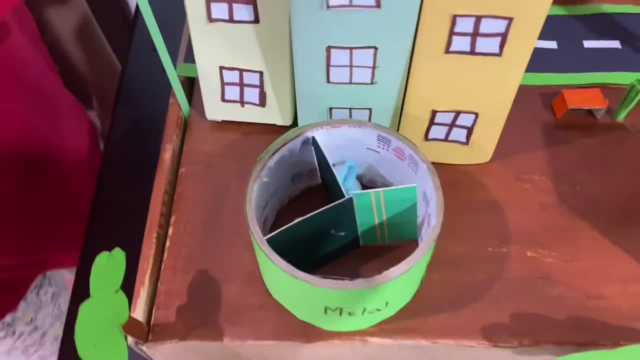 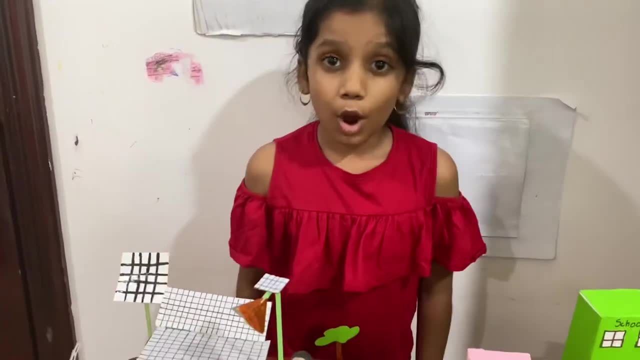 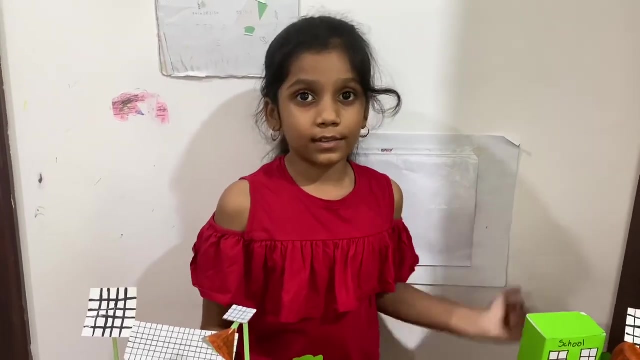 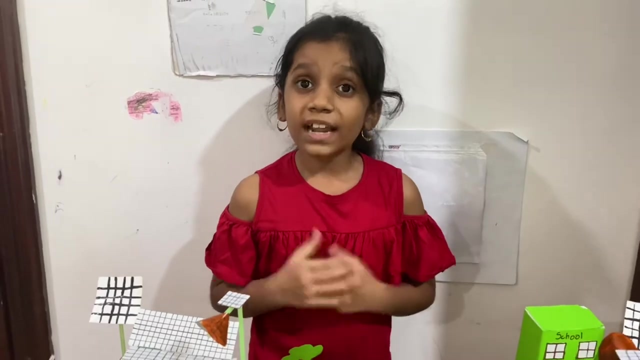 So that is theicy burn. It has three parts: metal, plastic and paper. This way, we can avoid separating the waste and this can be directly sent to the recycling centre. By planning the city this way, we can encourage people using public transport, walking or cycling. 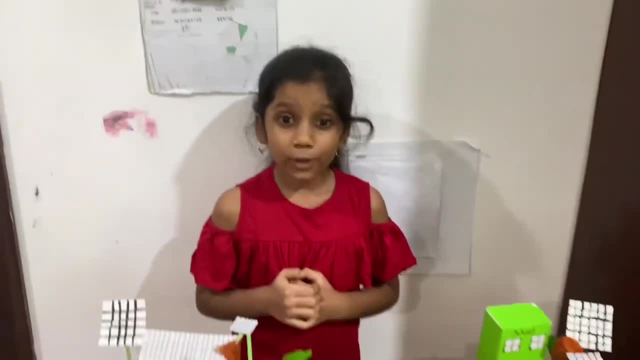 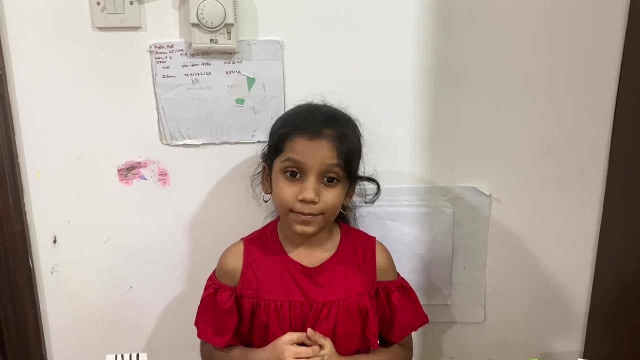 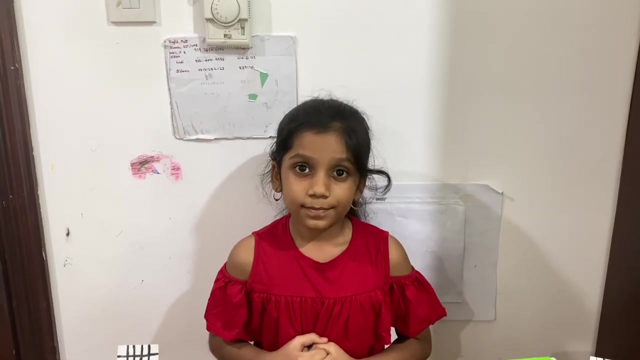 Do you know, aeroplanes also cause air pollution. We can book tickets in fly green, which will offset the pollution by planting trees. Thank you, Bye, See you in the next challenge. 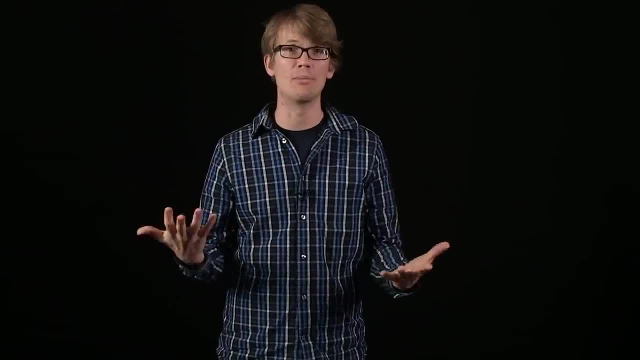 There's a lot of ideas that we just assume that we know a lot about because we hear about them all the time. For instance, I know what pop music is, but if you were to corner me at a party and say, Hank, what is pop music? 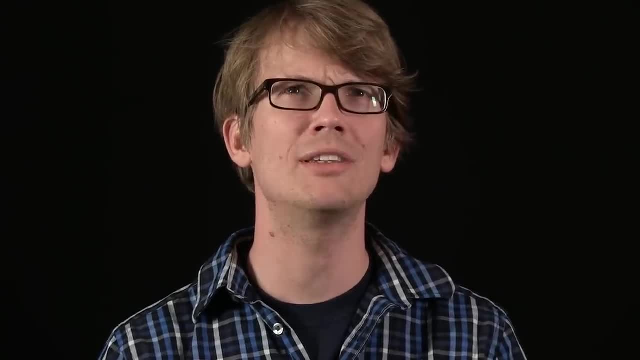 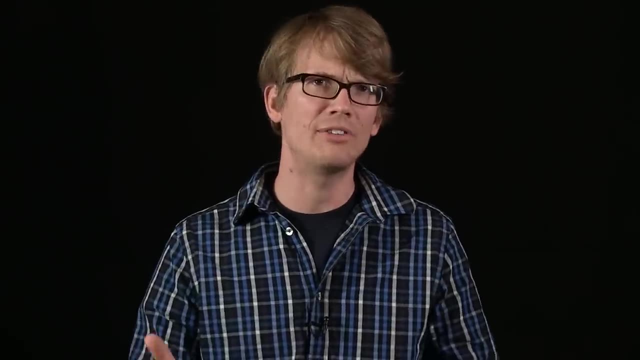 I'd be like it's uh. it's like, uh, the music that plays on the pop station. Just because we're familiar with a concept does not mean that we actually understand it. Ecology is kind of the same way, even though it's a common, everyday concept. 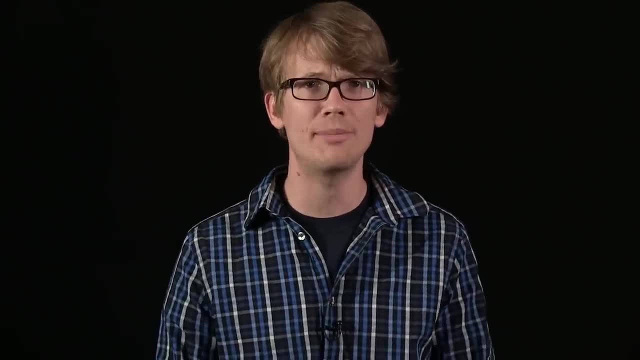 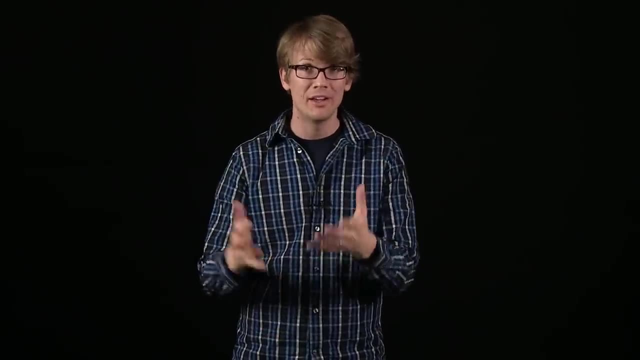 and ecosystem is a word that we hear a lot. I think most of us would be a little stumped if somebody actually asked us what an ecosystem is or how one works, or why they're important, et cetera. I find it helps to think of an ecosystem: a collection of living and nonliving things. 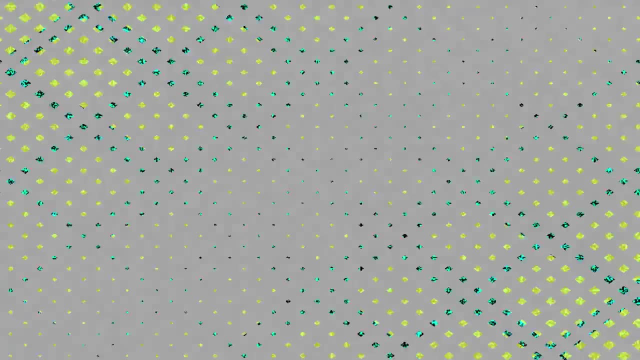 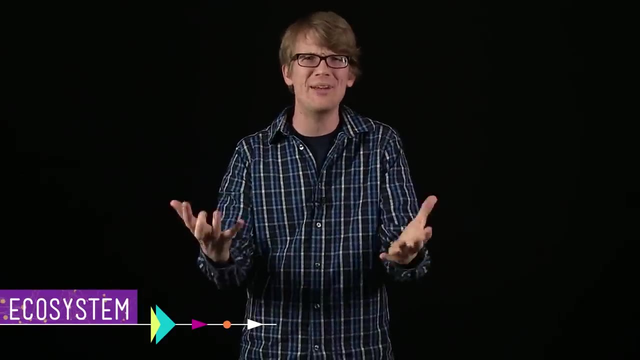 interacting in a specific place, as one of those Magic Eye posters for those of you who were sentient back in 1994.. An ecosystem is just a jumble of organisms and weather patterns and geology and other stuff that don't make a lot of sense together until you stare at them long enough.